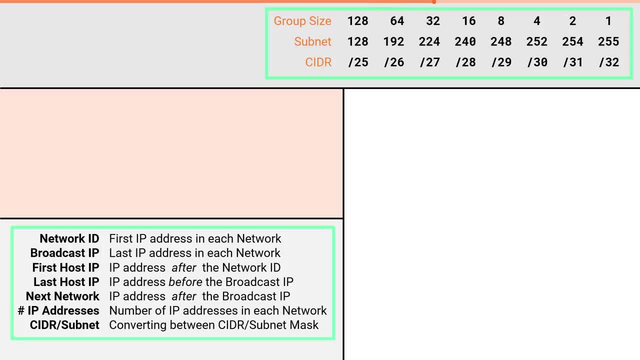 If you want to know the three steps to create this table, please check out video 2.. In this video, we will show you how to use the cheat sheet to solve all seven attributes for any combination of IP address and mask in 60 seconds or less. 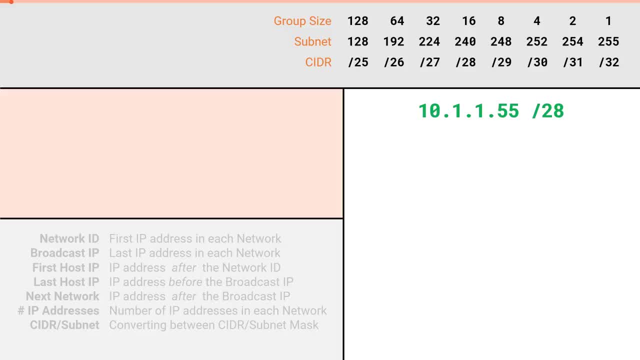 Our first example problem will be 10.1.1.55.28.. We will find all seven attributes for this IP and mask. We will start by learning how to quickly convert from a CIDR notation to subnetting problems. Our example problem provided a CIDR notation of slash 28.. 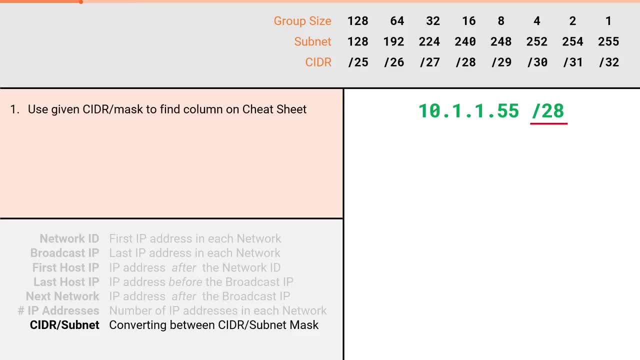 We will use that to find our column in the cheat sheet, Since we were given a slash 28,. this puts us in this column. Within our column, the CIDR row will map to the subnet row. The CIDR notation slash 28 will map to the subnet value of dot 240, which means our subnet mask will be 255.255.255.240. 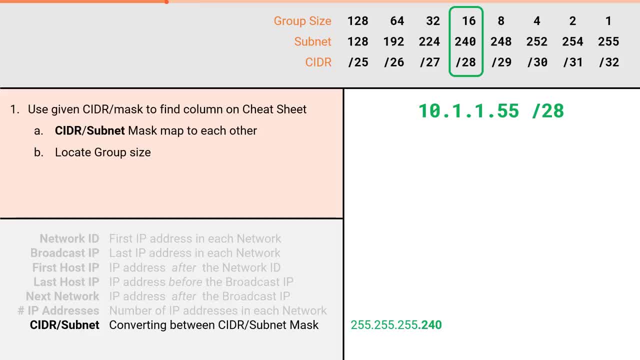 Next we will locate the group size For our problem with a slash 28,. the subnet value will be 255.255.255.240.. The group size will be 16.. Then we will start at dot 0 and continue incrementing by the group size until we pass the target IP. 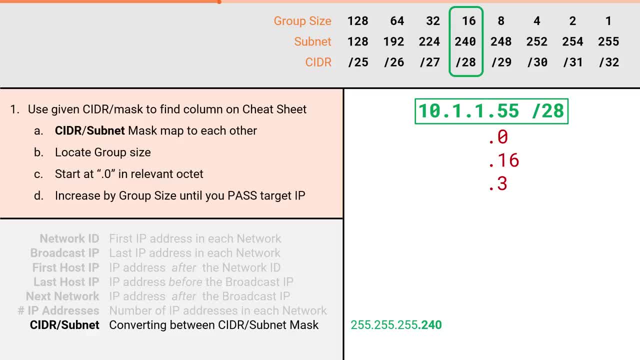 So we will have dot 0,, dot 16,, dot 32,, dot 48,, dot 64. And at this point we've passed our target IP of dot 55.. The dot 55 would exist somewhere between these two numbers. 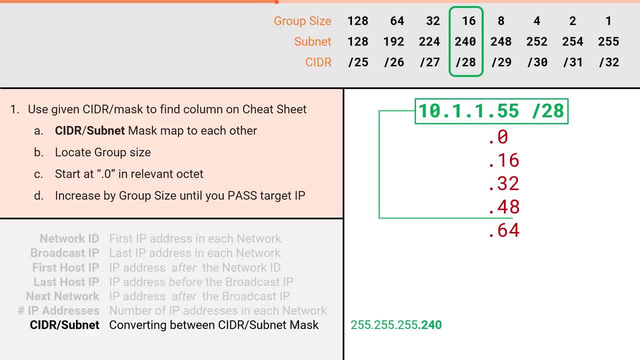 What we just did was the hardest part. From here, we can simply fill out the remaining attributes. The number before our target IP is our network ID. This makes our network ID 10.1.1.48.. The number after our target IP is our next network. 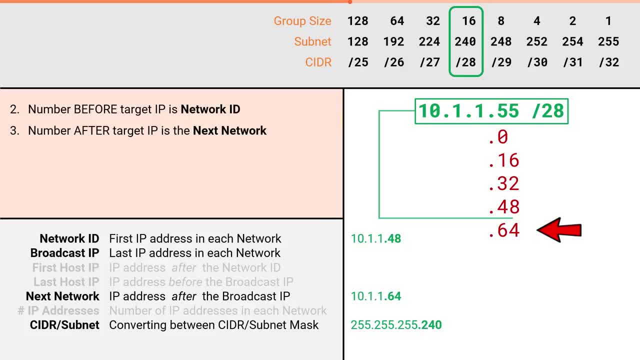 This makes our next network 10.1.1.64.. The IP address before our next network is our broadcast IP. This makes our broadcast IP 10.1.1.63.. Just like that, we were able to easily solve for three more. 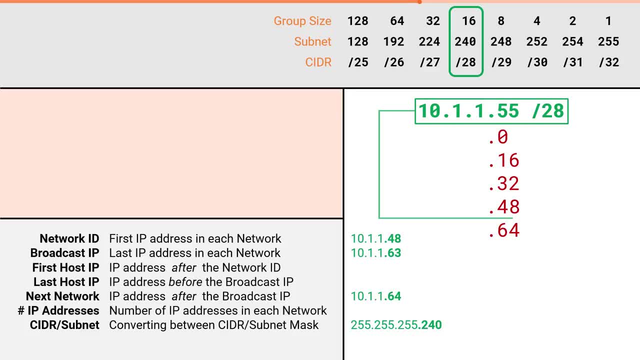 with the number of the seven attributes. Solving for the last three will be just as easy. To find our first host IP, simply add one to the network ID. If dot 48 was our network ID, then our first host must be 10.1.1.49.. 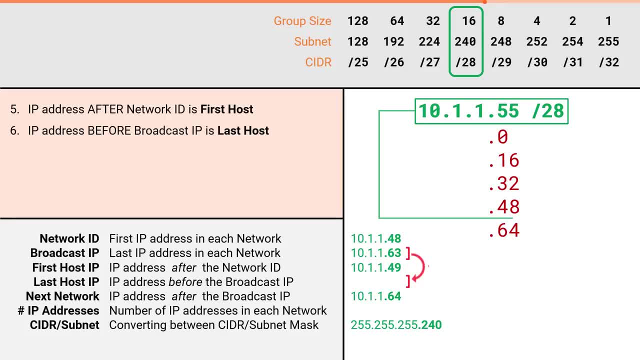 To find the last host IP, simply subtract one from the broadcast IP. If dot 63 was our broadcast IP, then our last host must be 10.1.1.62.. Finally, the number of IP addresses is very easy. The number of IP addresses is the same as the group size. 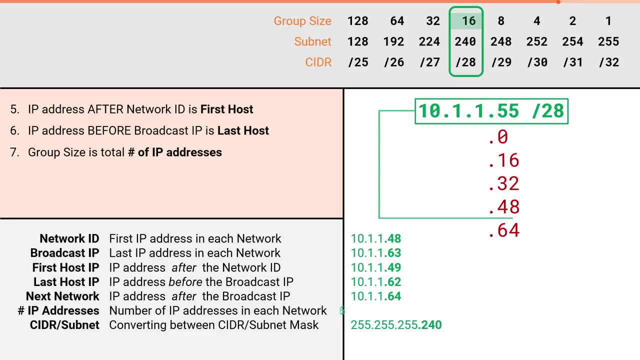 For r slash 28,. the number of IPs is 16.. Keep in mind, this is the total number of addresses. Remember that the network ID and the broadcast IP are not usable addresses. So if you're trying to solve for the number of usable addresses, 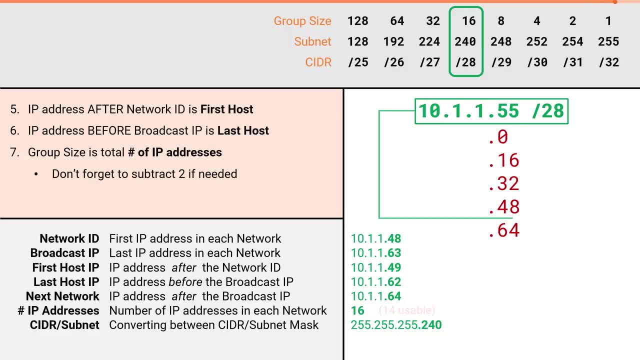 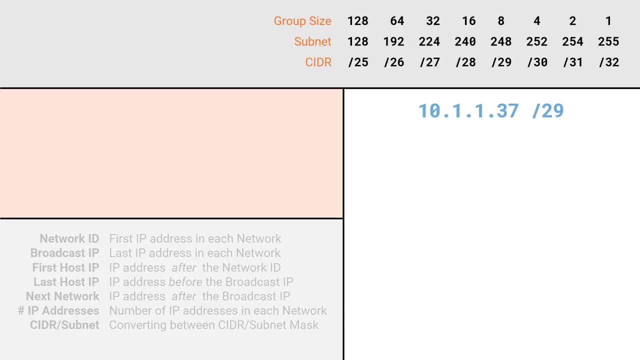 don't forget to subtract two For r slash 28,, we would have 14 usable addresses. We will run through the same process with another host. This time we will solve for all seven attributes for the IP and mask 10.1.1.37.29.. 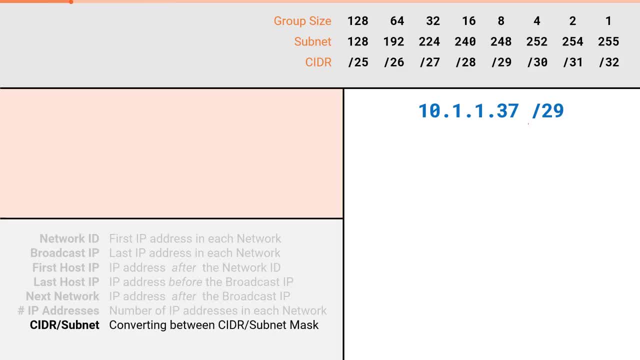 As before, we will start with converting between CIDR and mask. We were provided a slash 29.. We will use that to determine that we are in this column. CIDR and subnet mask rows map to each other, So we know that a slash 29 maps to dot 248,. 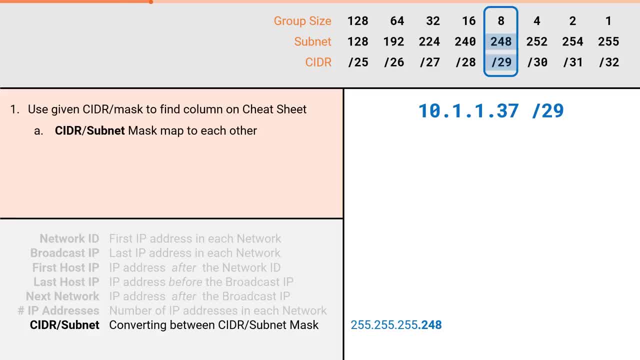 which gives us a subnet mask of 255.255.255.248.. Then we will locate our group size, which for this problem will be 8.. As before, we will start with dot 0 and increment by the group size until we pass the target IP. 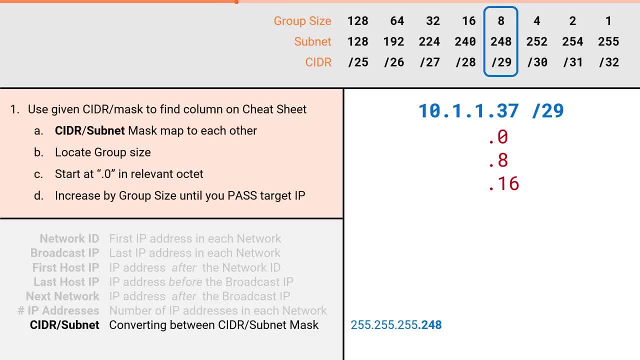 Dot 0,, dot 8,, dot 16,, dot 24,, dot 32,, dot 40.. We've now passed the target IP, so we can stop there. Dot 37 will exist somewhere in here. Once again, this was the hard part. 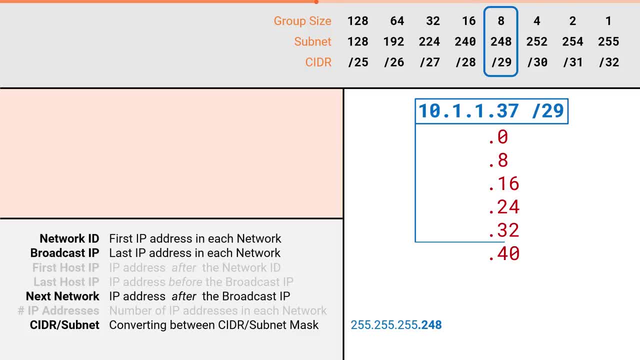 From here we can just fill everything in. The number before our target IP is our network ID. This makes our network ID 10.1.1.32.. The number after our target IP is our next network. This makes our next network 10.1.1.40..